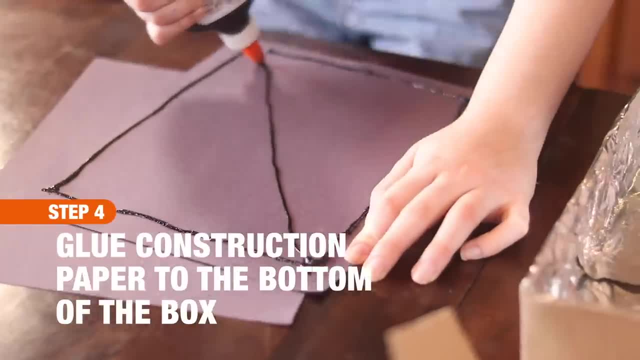 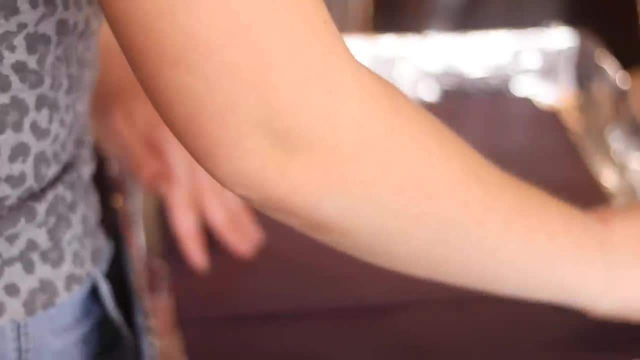 Next, take two pieces of black construction paper and glue them to the bottom of the pizza box. In place of glue, you could also use black duct tape. We use black construction paper because it's going to absorb the heat from the sun the best. 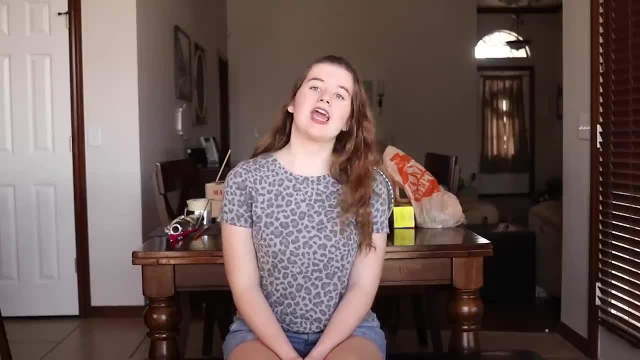